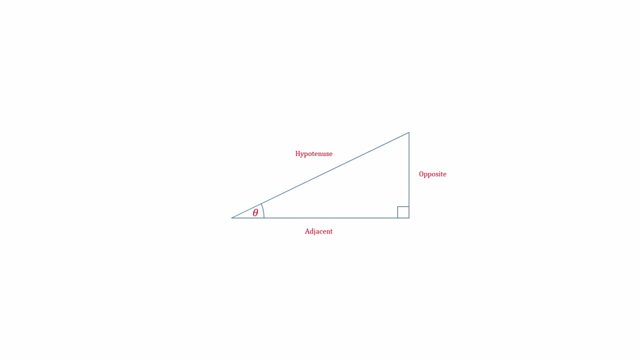 called the adjacent side, And this side, which is opposite the angle theta, is called the opposite side. Trigonometry tells us that the sine of angle theta is equal to the length of the opposite side divided by the length of the hypotenuse. 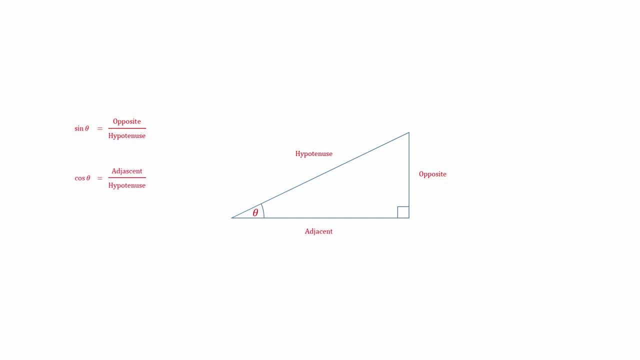 The cosine of angle theta is equal to the length of the adjacent side divided by the length of the hypotenuse, And the tangent of theta is equal to the length of the opposite side divided by the length of the adjacent side. These formulas are incredibly useful If we know the angle theta and the length of one side. 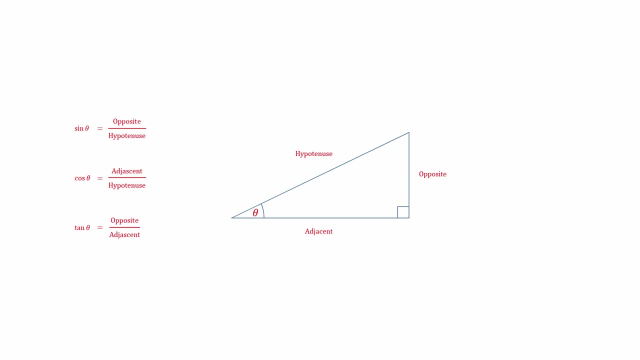 we can calculate the lengths of the other two sides, Or if we know the length of two sides, angle theta or the length of the other side. For example, suppose you're standing 50 meters away from a tall tree and you use a sextant or just a protractor and a 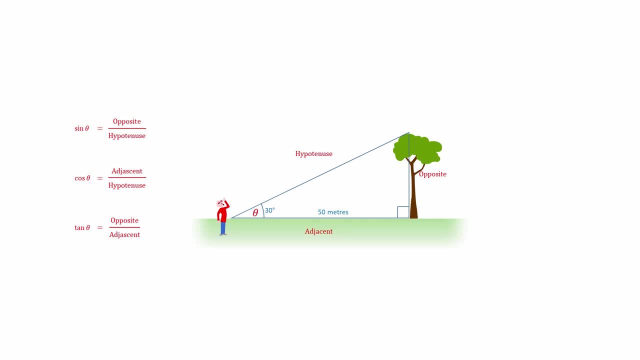 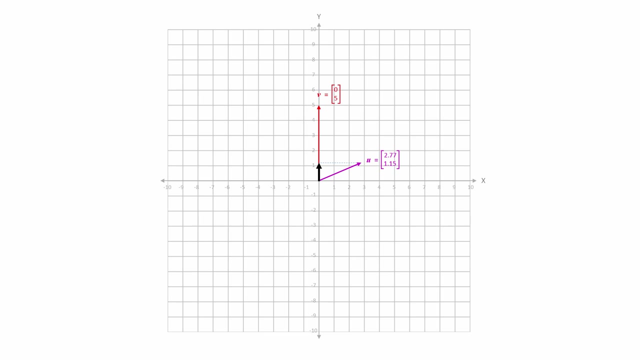 piece of string to measure the angle between the ground and the top of the tree. You can calculate the height of the tree without having to climb up it like this. Let's zoom in and take a closer look at these vectors and see how trigonometry can be applied to calculate the angle between them using only the 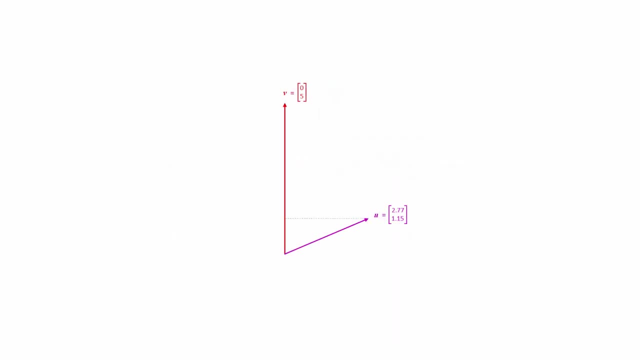 information you can see here. First, label the angle you want to find as theta. Notice that the short vector and its orthogonal projection form two sides of a right angle triangle. We already know that the length of the tree is the length of the tree. 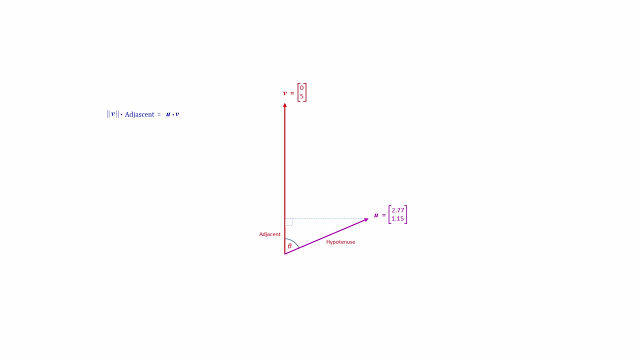 that the length of vector V multiplied by the length of the projection is equal to the dot product of the two vectors. This can be rearranged to give an expression for the length of the adjacent side. Now, given that the cosine of theta is equal to the length of the adjacent side divided by the length of, 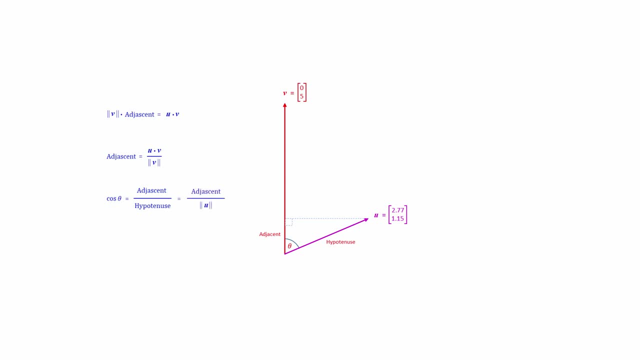 the hypotenuse, then the cosine of theta is equal to the length of the adjacent side divided by the length of vector U. When these two expressions are put together, we arrive at a formula that can be used to calculate the angle between two vectors. Let's give it a try. First, calculate the dot product of the two.